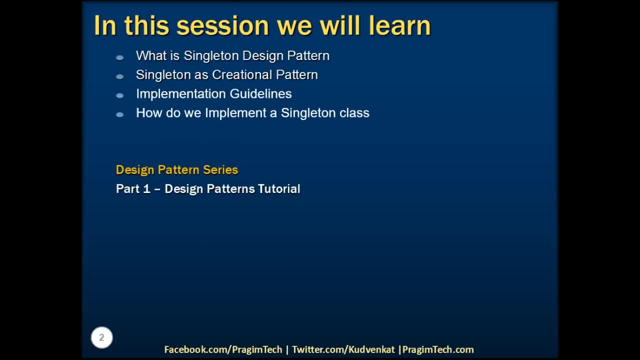 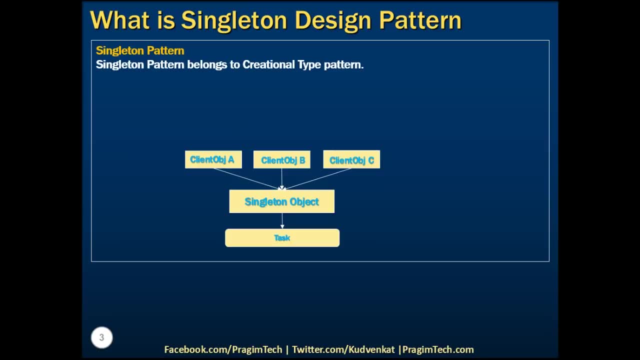 This is continuation to part 1 of the Design Patterns tutorial, So please watch part 1 before proceeding. Singleton Pattern belongs to Creational Type Pattern. Let's recap what is Creational Design Pattern. As mentioned in the part 1 of the tutorial, Gang of 4 have identified 5 design patterns that belong to Creational Design Type category. 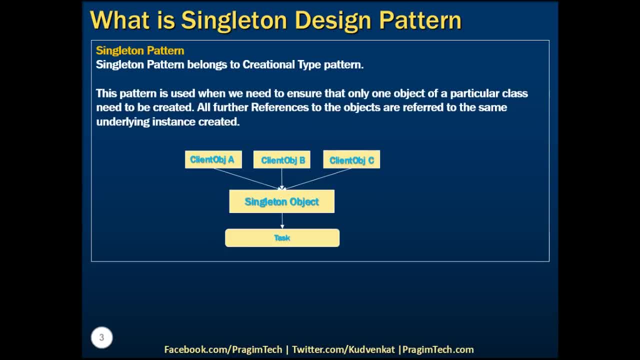 Singleton is one among them, and the rest are Factory Abstract, Factory Builder and Prototype Patterns. As the name implies, Creational Design Type deals with the object creation mechanisms. Basically, to simplify, this Creational Pattern explains us the creation of objects in a manner suitable to a given situation. 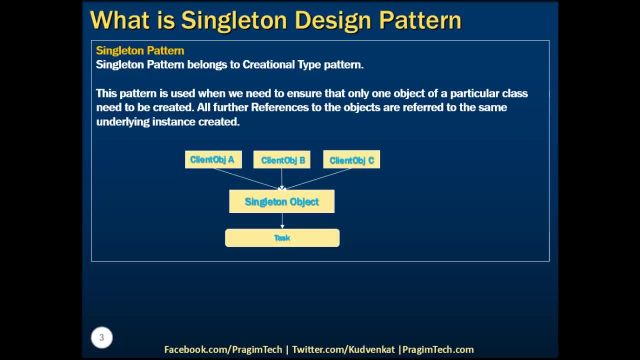 I hope now you are familiar with Creational Type Pattern. Let's now focus on Singleton Design Pattern. Singleton Design Pattern is used when we need to ensure that only one object of a particular class is instantiated. That single instance created is responsible to coordinate actions across the application. 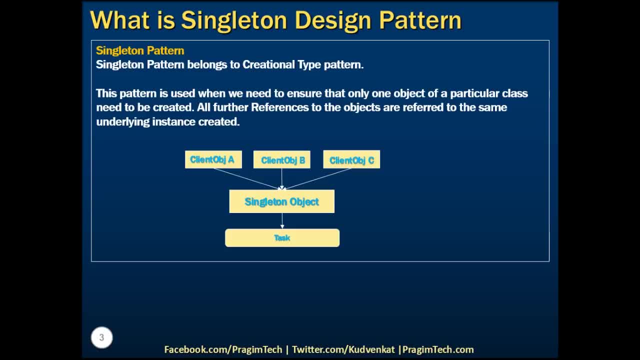 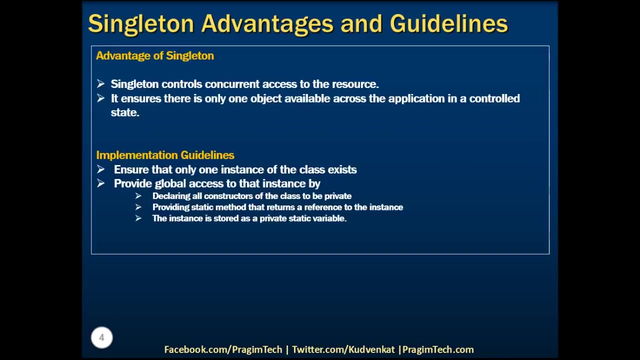 If you look at the illustrated diagram, you will see different objects trying to invoke an object instantiated as Singleton. This single instance of the object is responsible to invoke underneath methods or events. Let's look at advantages and guidelines in Singleton implementation. Concurrent access to the resource is well managed by Singleton Design Pattern. 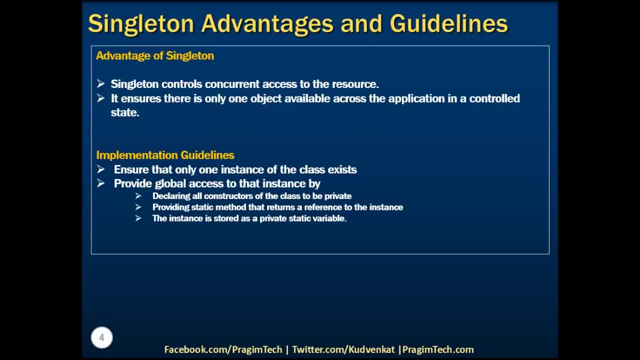 As part of the implementation guidelines, we need to ensure that only one instance of the class exists by declaring all constructors of the class to be private. Also, to control the Singleton access, we need to provide a static property that returns a single instance of the object. 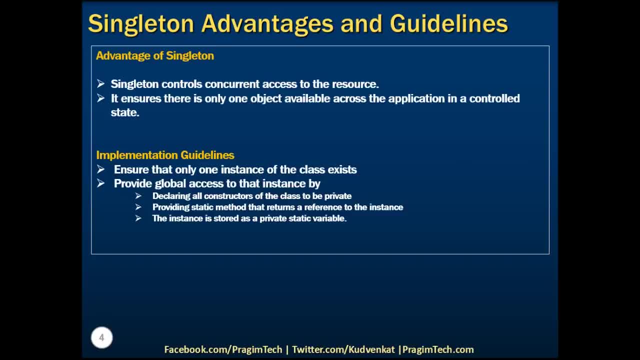 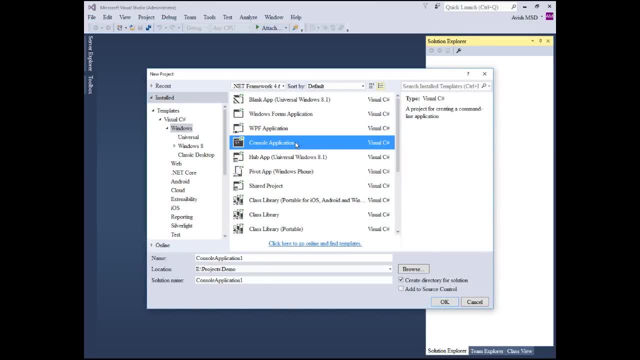 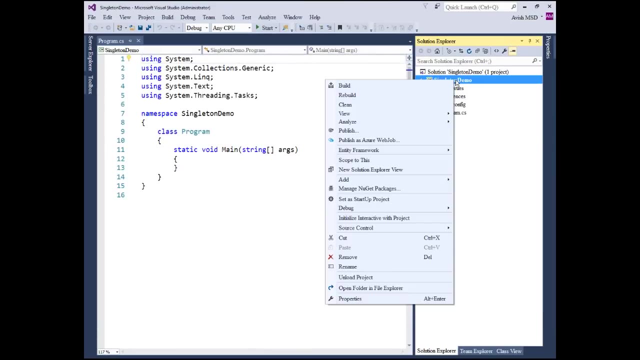 Now let's flip to Visual Studio and see this in action by implementing a Singleton class. Let's create a new project and choose Console application. Let's name this as SingletonDemo. Let's add a new class. Name it as Singleton. Let's create a public method. 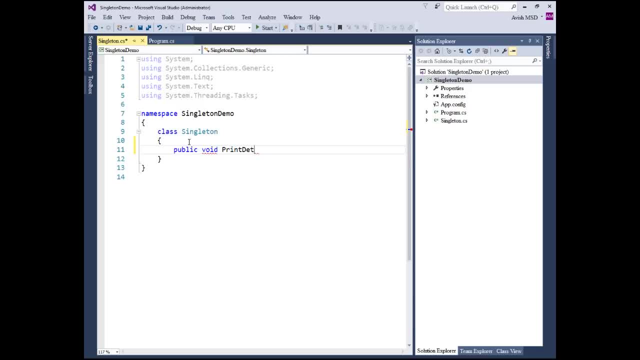 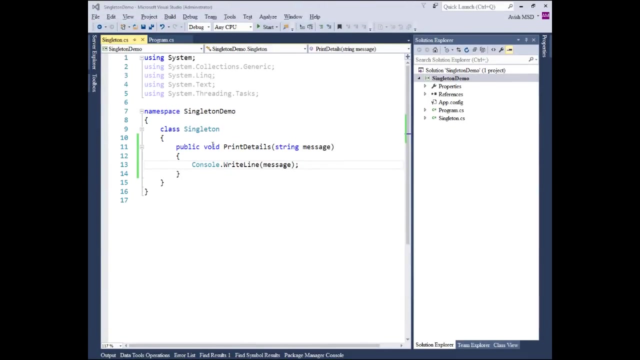 public void printDetails which accepts string as the input parameter. Let's just print this message using your consolewriteline. Let's just compile this. For our convenience, we have named this class as Singleton. We have not yet applied any Singleton design pattern principles to this class. 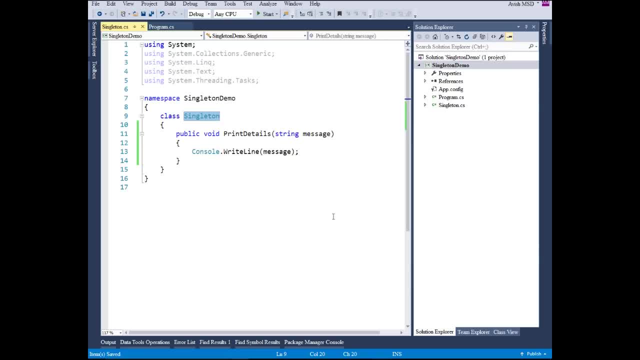 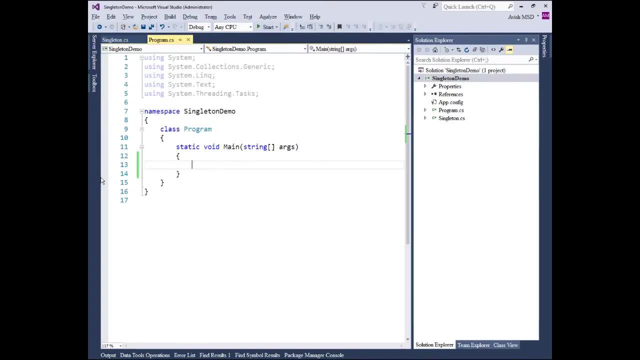 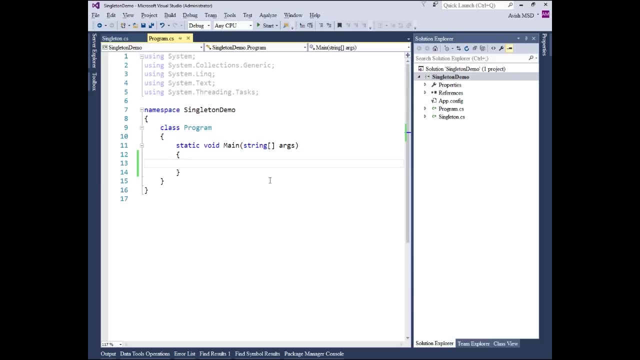 Let's see why we need to apply Singleton design principles and how we can apply them for this Singleton class. Now that we have created a Singleton class with printDetails as a public method, we can invoke that public method from this main program by creating a new object of Singleton. 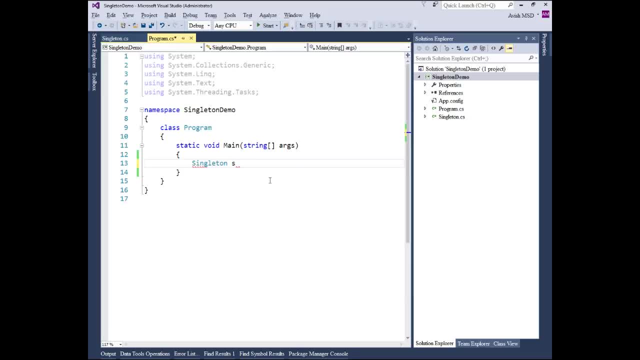 Let's see how to do that. Singleton s1 is equal to new Singleton, and then s1.printDetails. Let's just say this is first message. If we want to print another message, we just need to say s1.printDetails again. 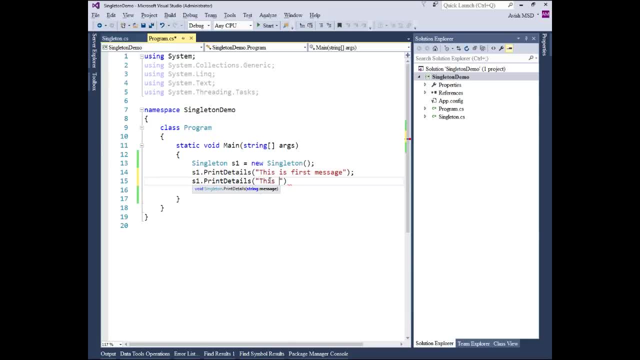 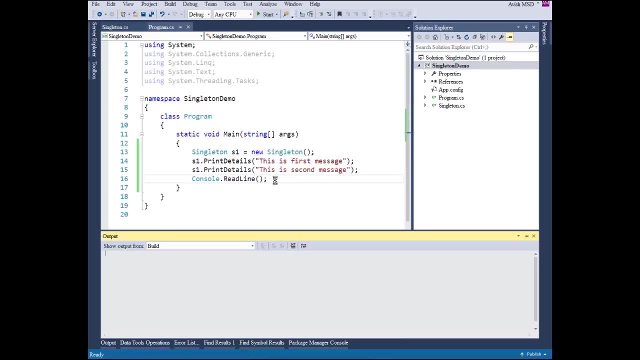 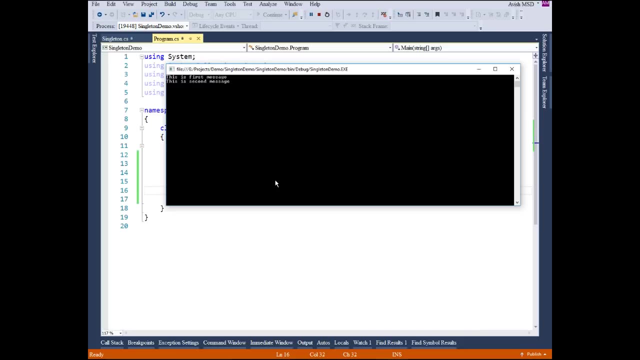 This time let's say: this is second message. Let's compile this, Let's run this program. Look at that. The program has outputted two statements. This is first message and this is second message. That means we have instantiated only one object and we are able to invoke a printDetails method. 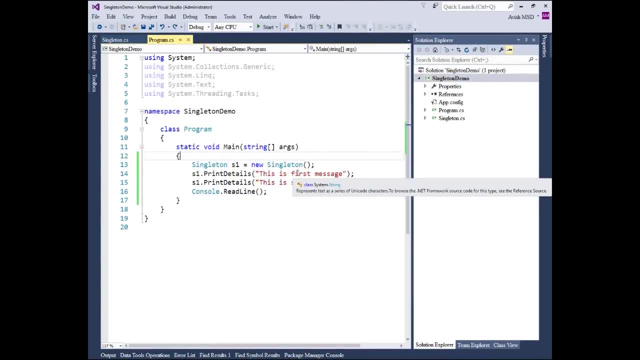 Imagine a situation where we need to invoke printDetails from different classes of a given project. What we do is we end up creating multiple objects of this Singleton class. Let's say we create the Singleton object for an employee, So let's just change this s1 to fromEmployee. 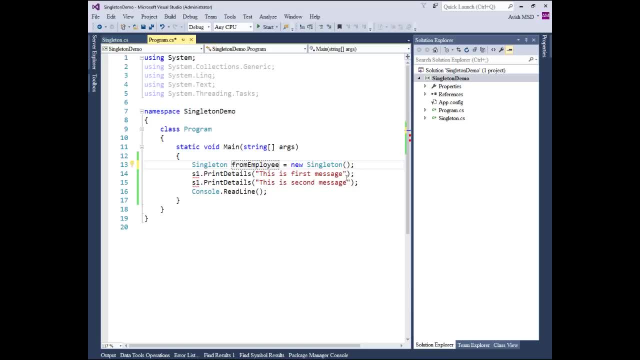 That means we are assuming that we are creating this object from an employee class And then say that employeeprintDetails, And let's change this message as fromEmployee, And then let's assume that we need to invoke this Singleton object from a student class. 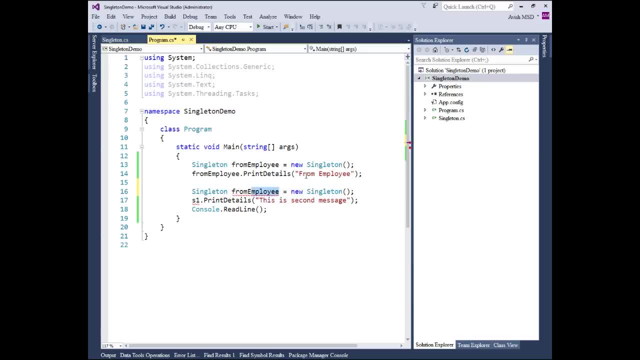 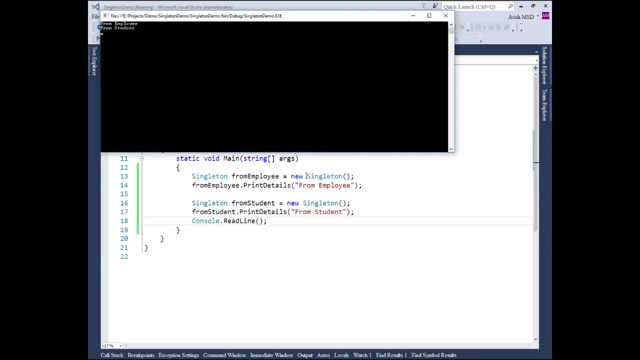 We would say from student, And then let's print the details from student And let's pass the message as from student. Let's compile this Compilation succeeded and let's run this program. Look at the output. The output has printed a message from employee and from student. 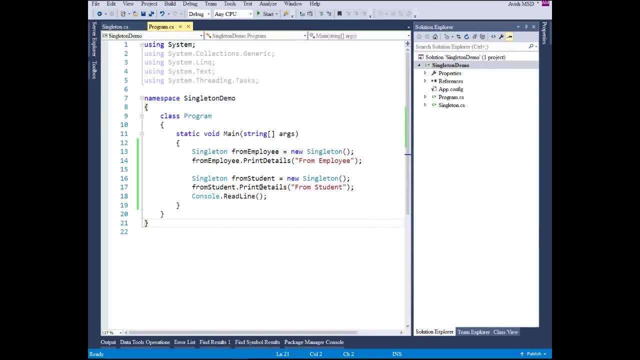 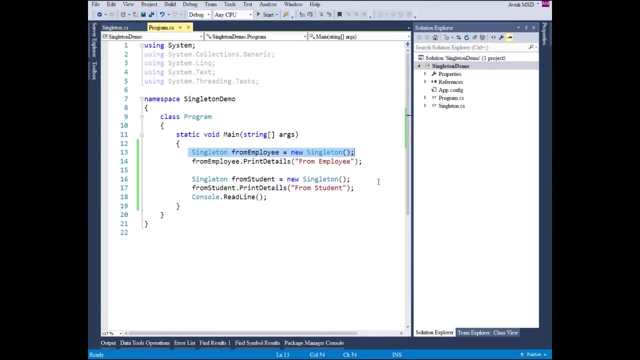 This means, whenever we need to create an instance of Singleton or invoke the printDetails method of Singleton, we end up creating multiple objects. Let's prove that it has created multiple objects. How do we do that? Let's go back to the Singleton class. 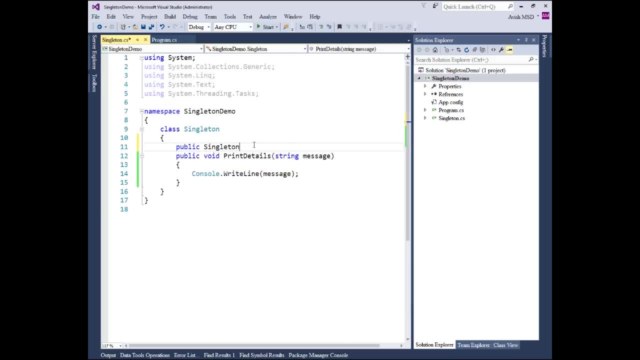 Let's add a public constructor called Singleton And then let's create a private static incremental variable. We will be incrementing the counter as and when a new instance is created using the Singleton class. Now, once we increment the counter, let's output the counter value using our consoleWriteLine. 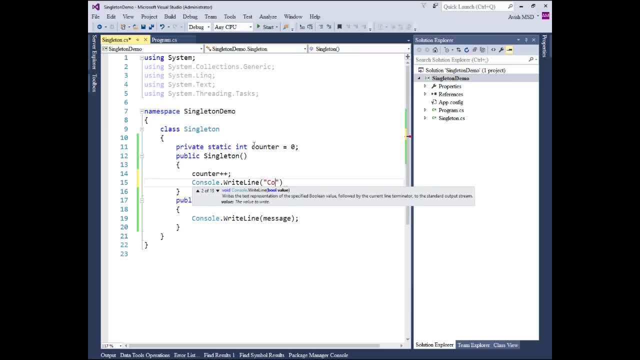 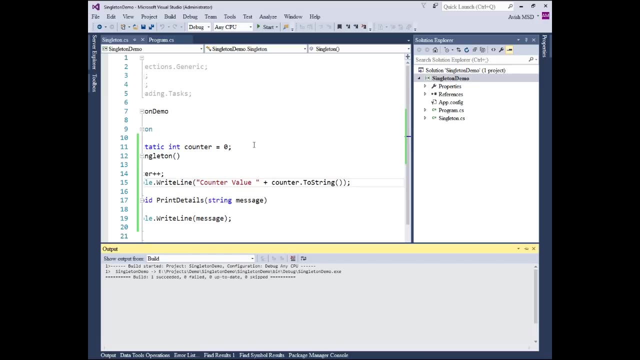 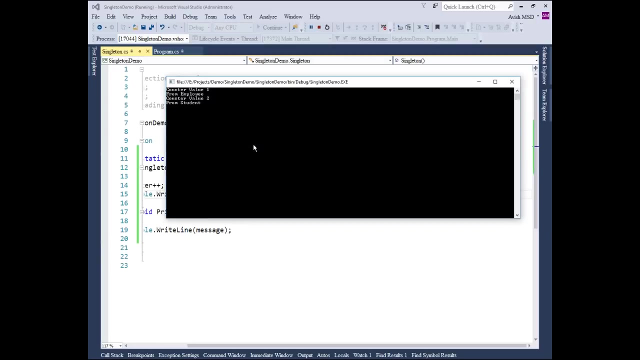 And say counter. Counter value is counterToString. Let's compile this application and run this again. Look at that. We ended up creating two instances of Singleton class, which is evident from the counter value too. That means first time when we create the Singleton object from employee, the counter value is incremented to one. 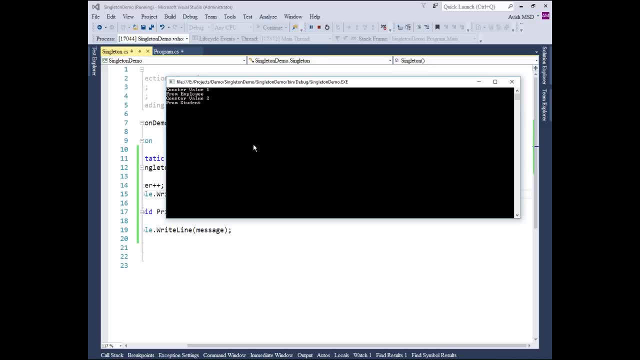 And second time, when we create another instance of the Singleton object, the counter value is incremented to two. Even though we are invoking a very common method, we are ended up creating two instances of the same Singleton class as objects. Now that we have proved it's unnecessary to create new instance of Singleton class, 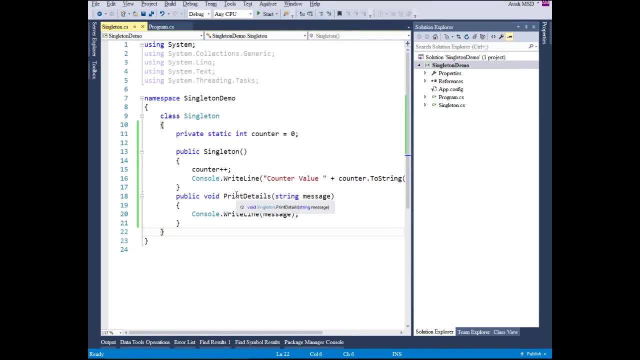 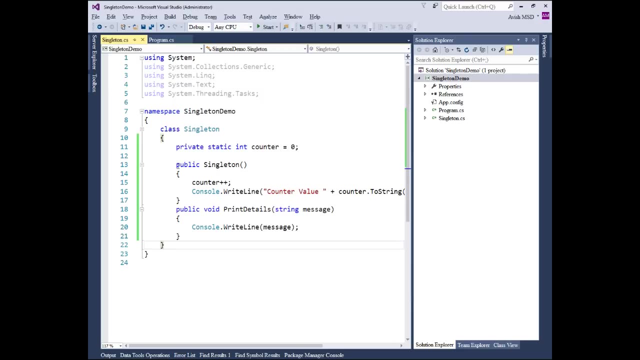 Let's see how we can avoid that. The first point comes into mind is to restrict the multiple instance creation. We can achieve it by making all constructors as private and change the class to sealed class, so that it's not inherited anymore. Let me change this public constructor to private. 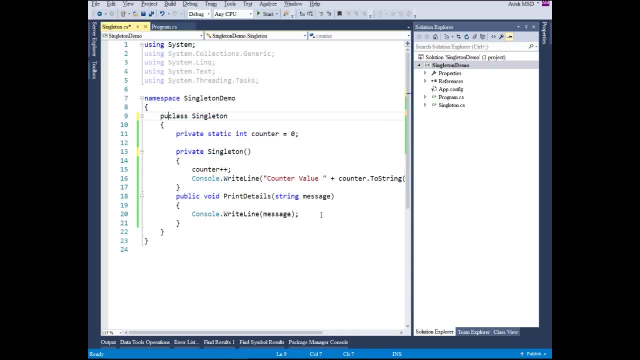 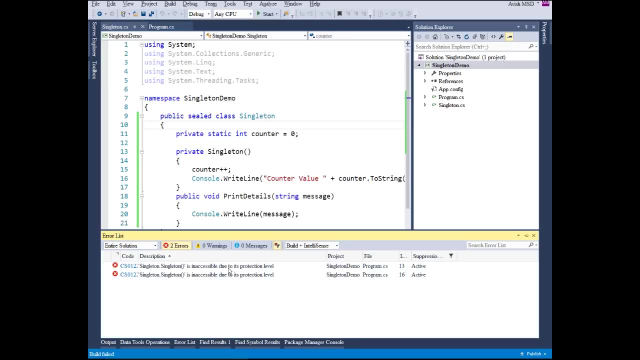 And let's also make this class as sealed class, As Singleton. Let's compile this application now and see the behavior. Look at the error messages here. It says the Singleton is inaccessible due to its protection level. Let's see where it is throwing the error. 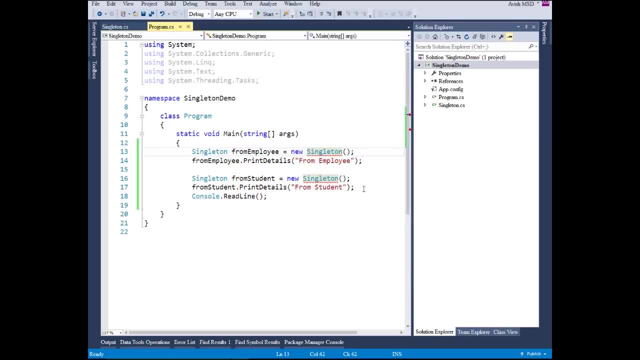 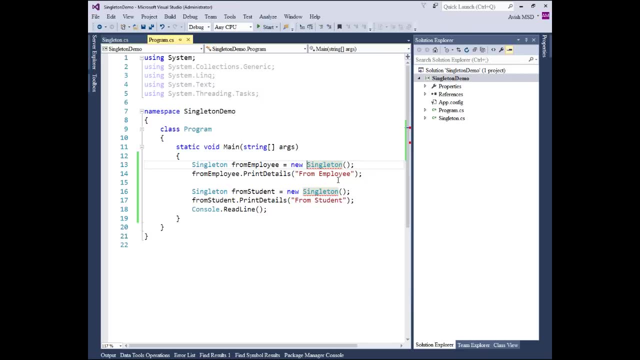 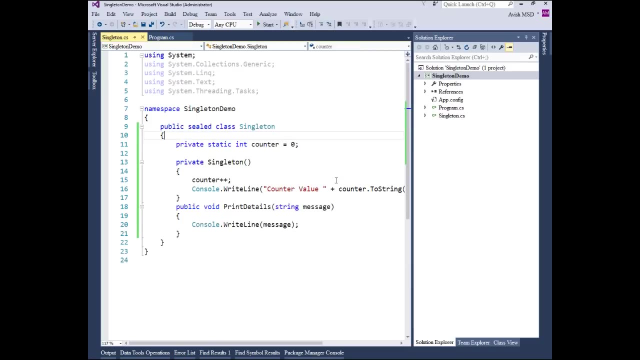 Look at that. For every new object instantiation it is throwing an error. right now That is because we have changed the public constructor into private, So we are not able to instantiate the class. When we are not able to instantiate the class, we need to provide an alternative way where we can give back the Singleton object creation. 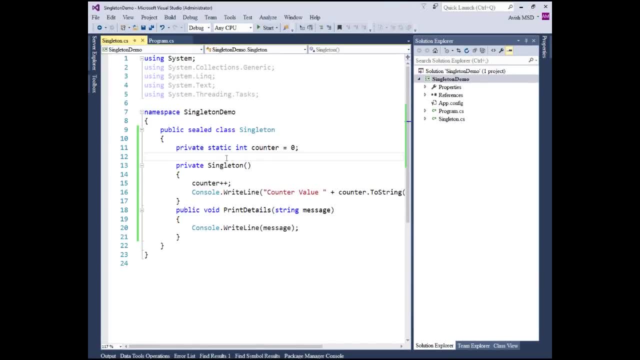 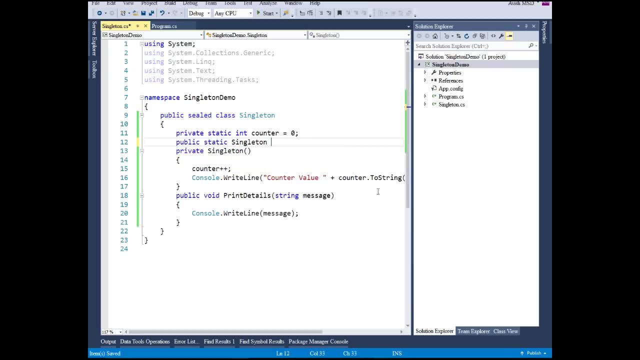 Let's see how we can create a single instance of this Singleton class. Let's create public static Singleton. Call it as get instance. Return new Singleton. Look at that. We have not overcome the problem of creating multiple instances if we return new Singleton instance in this get instance property. 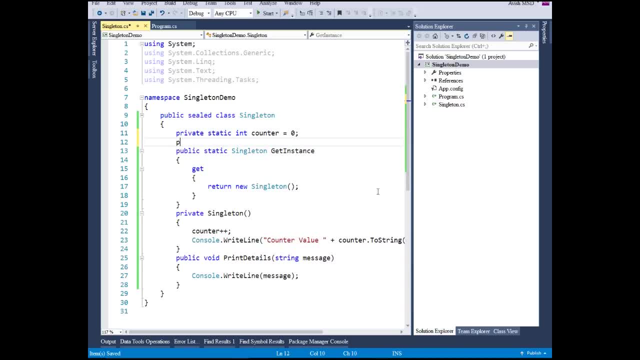 How do we avoid this? Let's create a new private static Singleton. Let's call it as instance, which is equal to null. We need to create an instance only if the above declared private property is null. So let's put the check Instance equal to null. then instance is equal to new instance. 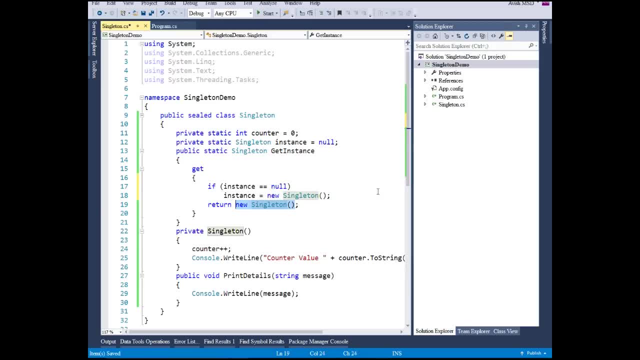 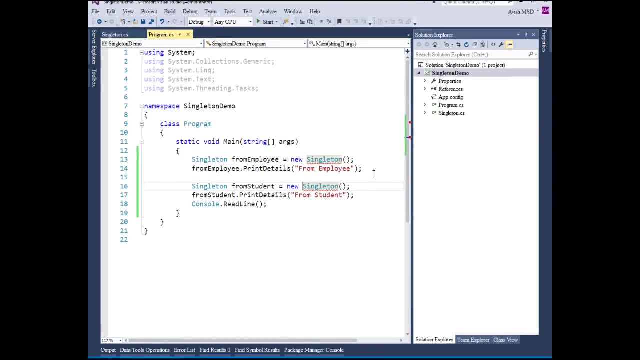 And then let's modify this code and return instance instead of new instance. With this, we have applied the Singleton design pattern to our Singleton class. Let's go back to the program and see if the error is gone. No, the error is not gone yet. 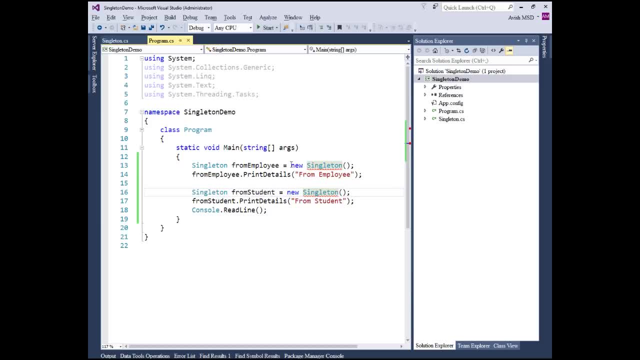 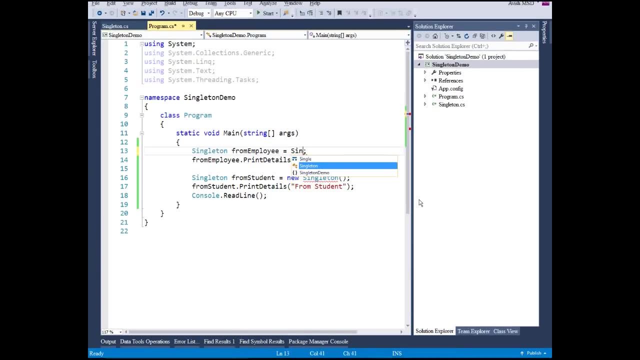 Reason: we are still trying to instantiate a new Singleton class. Let's change it. Instead of doing a new Singleton, Let's use the property which we have created, Which is the get instance. Let's say, instead of doing a new instance,